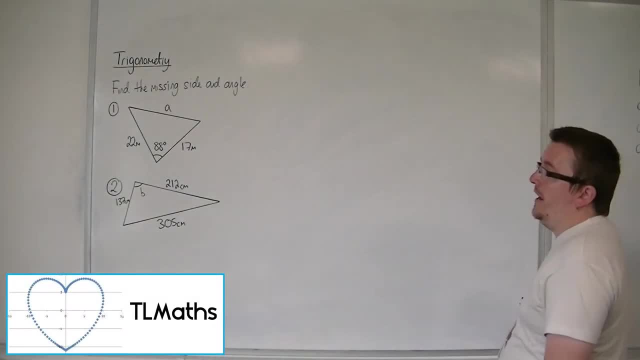 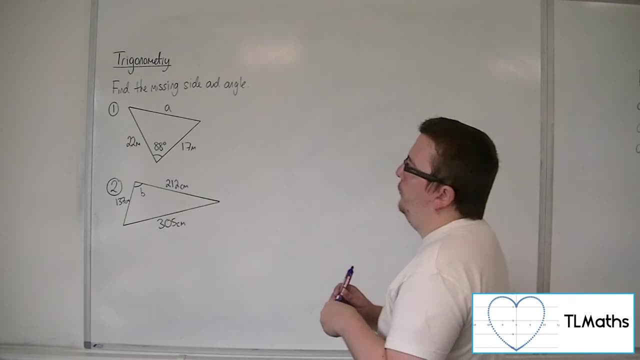 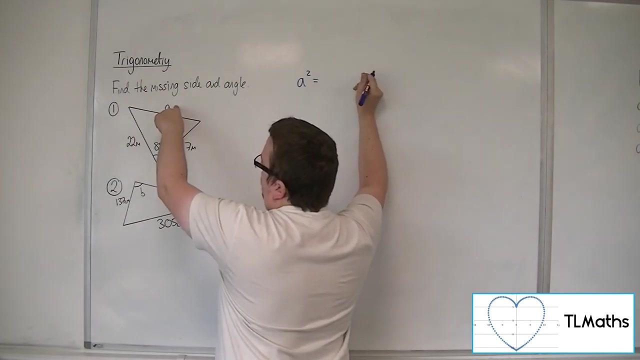 Okay. so let's say I want to find the missing side and angle in these two diagrams, Both of these. I'm going to have to use the cosine rule, okay? So for this first one we have that a squared. okay, so this side squared is equal to. now. either of these could be b and c, it doesn't matter which. 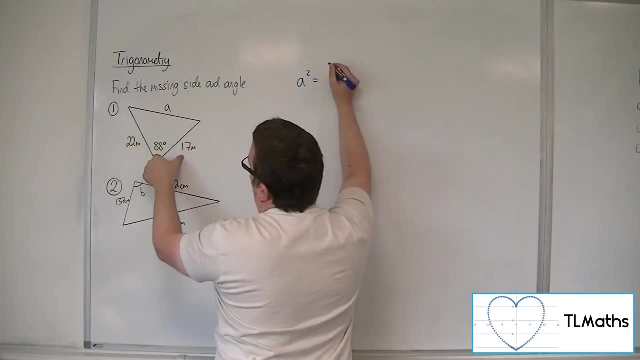 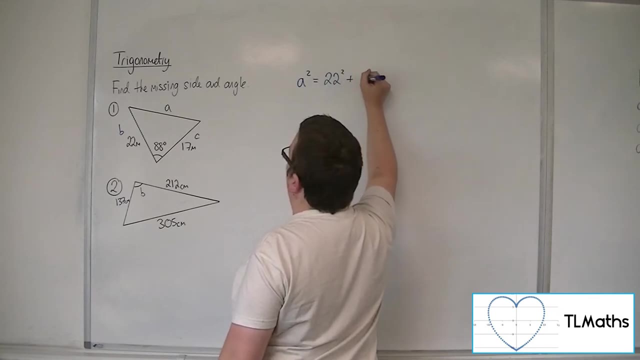 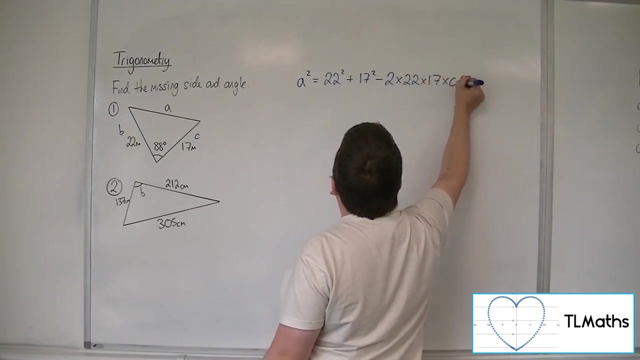 So let's go with: 22 is b, 17 is c. let's quickly label them. So we've got b squared, it's 22 squared plus c squared minus 2, lots of b times c, times cos of the angle 88 degrees. 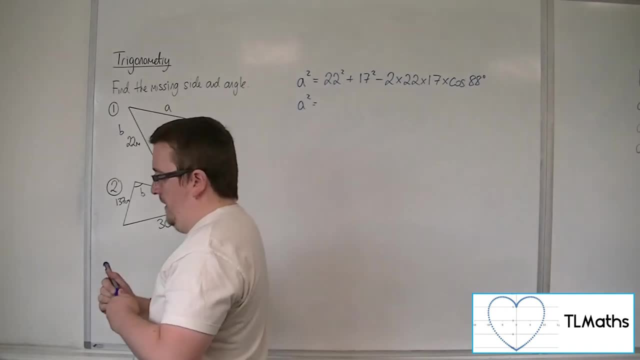 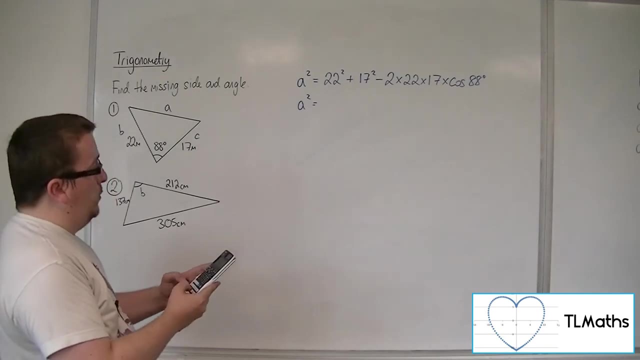 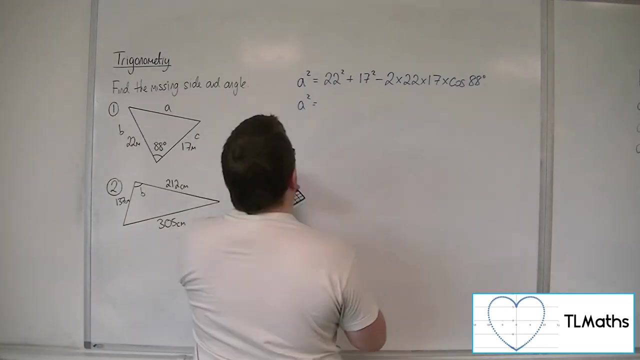 Okay, so a squared. I can just plug all of that straight into the calculator. So 22 squared plus 17 squared. take away 2 times 22,, times 17,, times cos, So the cosine of 88 gets me 746.895, etc. 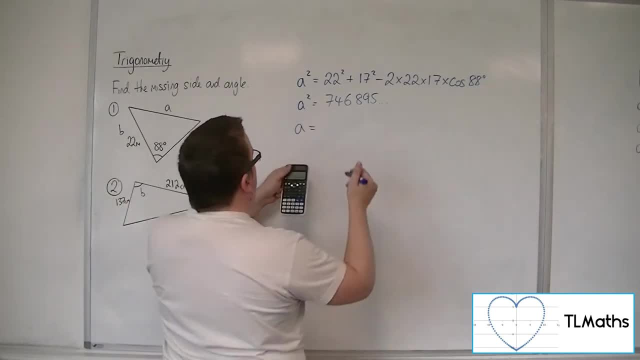 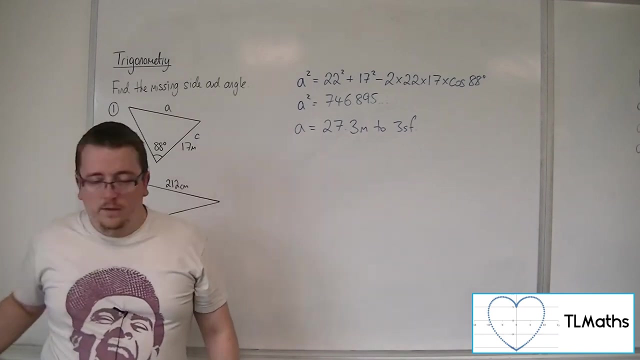 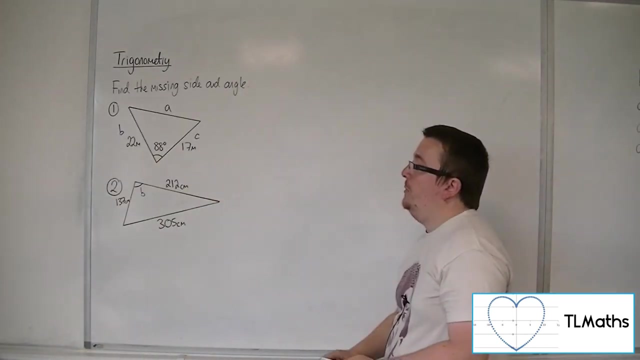 So then, square root alza key is 27.3 meters to 3 significant figures. okay, And so that is my answer to number 1.. Now number 2 requires, It requires me to find an angle. Now, depending on whether you actually remember the rearranged version of the formula or not, I'm going to say let's say we don't okay. 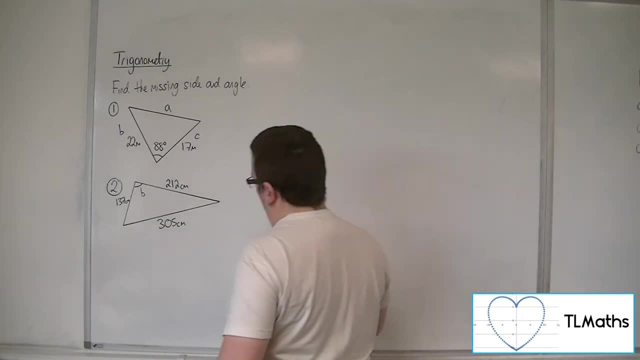 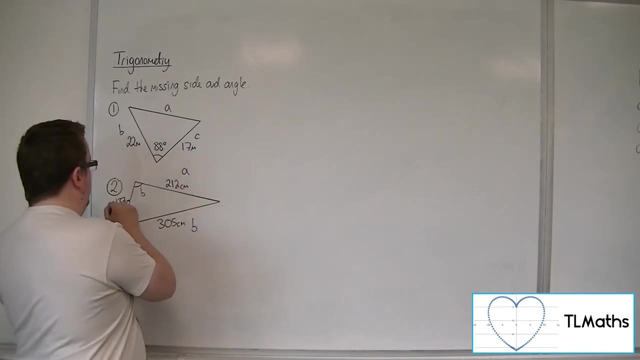 Let's say we don't know that, So that, well, we can call this one a, if you like, there's b and there's c, or probably even better, right, Rather than labeling it that, Let's call that angle a, there's little a, there's b, there's c, for example. 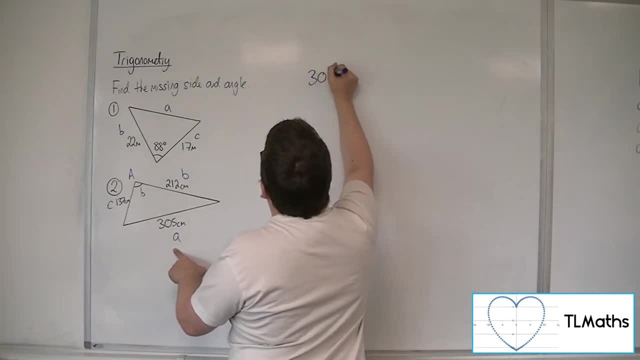 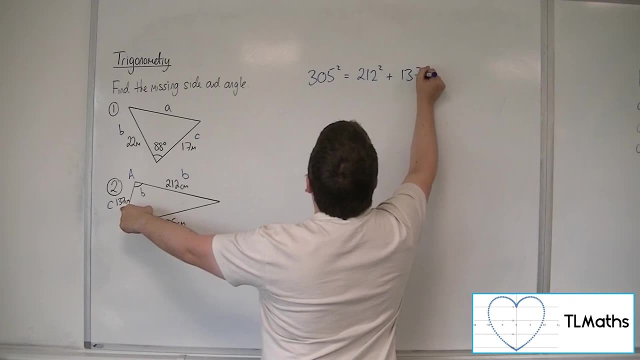 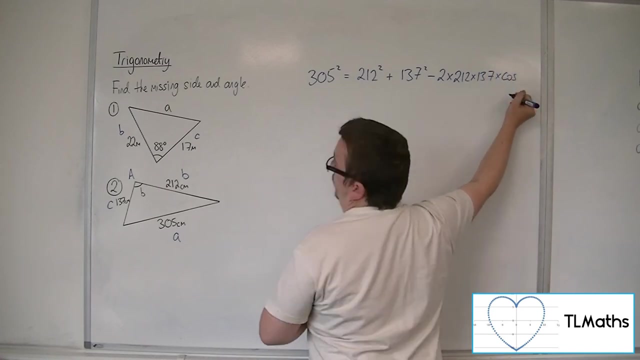